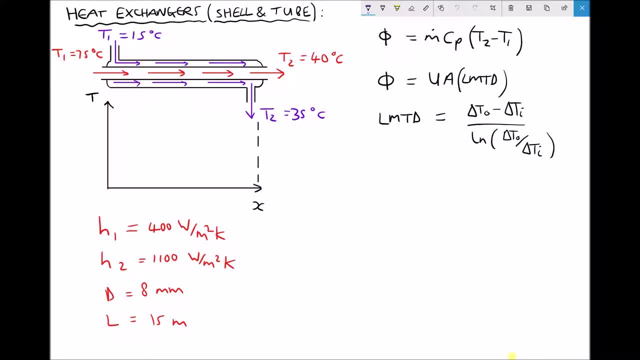 itself can be exactly the same in construction, and the type of heat exchanger drawn on the screen here is called a shell and tube heat exchanger. So from the diagram, we have a tube in the centre carrying a hot fluid and around the outside we have a shell or a water jacket. 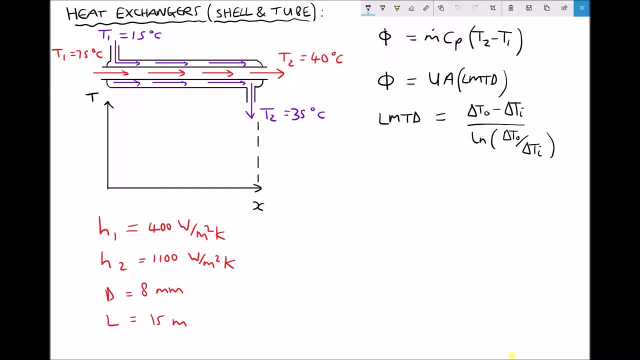 carrying the cold fluid. What we have drawn here is a single pass heat exchanger, so we've only drawn one tube and one shell, but in reality these heat exchangers can have a number of passes where the two fluids go backwards and forwards through the heat exchanger, which 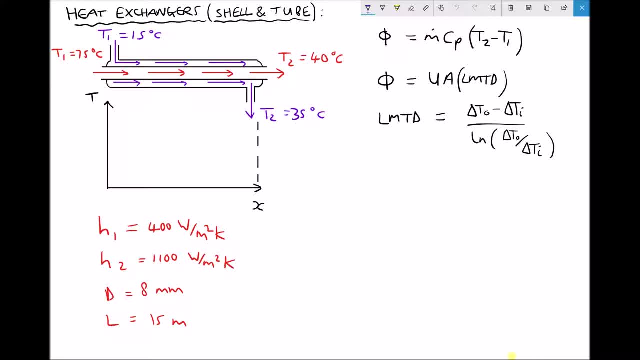 in effect increases the contact area. But we're going to keep things simple for this tutorial. Now, on the diagram, we've specified the inlet and outlet temperatures of our hot fluid as 75 degrees C and 40 degrees C respectively, and we've also specified the inlet and outlet. 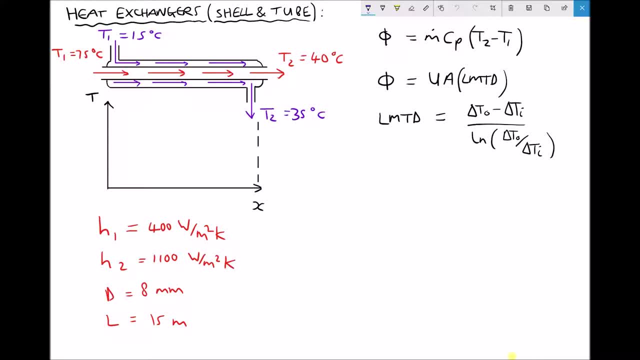 temperatures of our cold fluid as 15 degrees C and 35 degrees C respectively. In the bottom left hand corner I've also included some additional data. We have surface heat transfer coefficients for fluid 1 and 2 as they make contact with the outside surface of the heat. 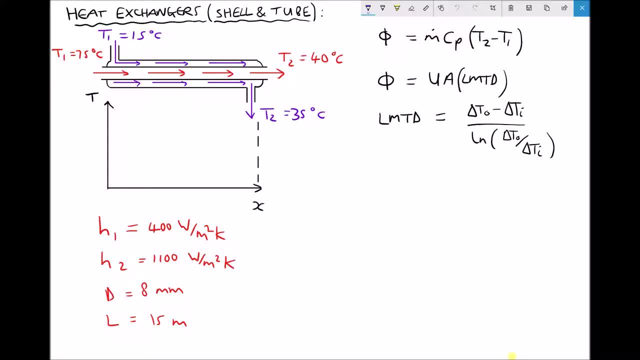 exchanger tube. What we're assuming here is that conduction through the walls of the heat exchanger is negligible when compared to the surface heat transfer effects, And in order for that to be true, the thickness of the walls would have to be negligible and the thermal 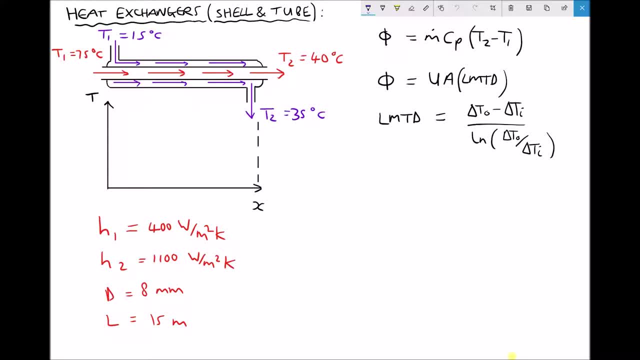 conductivity would have to be relatively high. Now, when we design heat exchangers, that's something that we try to do in the design of heat exchangers. We try to make sure that the heat exchangers are in the right temperature and that the heat exchangers are in the right 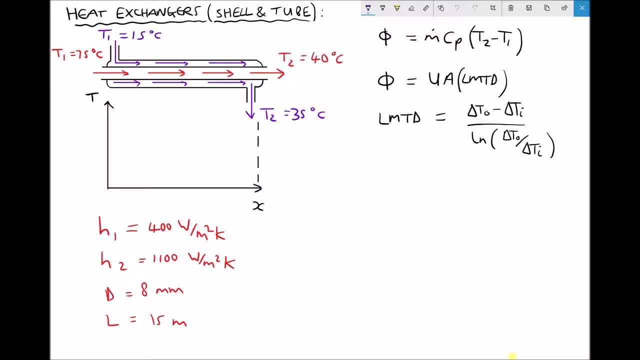 temperature in order to optimise heat transfer between the two fluids. So we have our two surface heat transfer coefficients. We also have the diameter of the tube and we have the length of the tube. Note that we only have one diameter and one length and 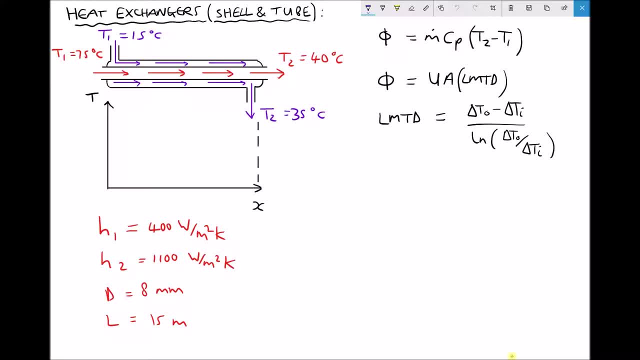 that will be for the tube running through the centre, because the contact surface area between the two fluids is the outside surface of that tube. The diameter of the shell itself is irrelevant, because contact between the two fluids occurs at the surface of the tube. So over on the right hand side, we have two different formulas for calculating rate of. 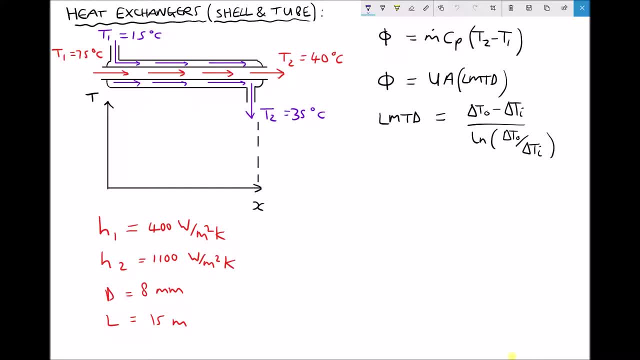 heat transfer, The one at the top. we've seen previously Mass flow rate times, specific heat capacity times, temperature change. But in the example we're looking at here we don't have a mass flow rate for the fluid and we don't have a specific heat capacity. So we're 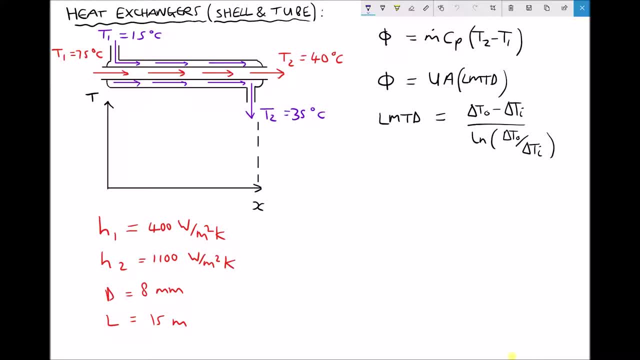 unable to use that particular formula. Instead, we're going to use the second formula, which states that rate of heat transfer equals UA times heat transfer times temperature change. So that's the first formula. Now, if we look, something called the log mean temperature difference. A is the contact area for the 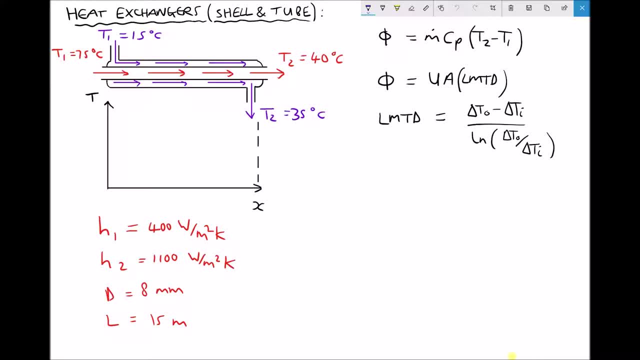 two fluids, as we discussed previously. U is the overall surface heat transfer coefficient and LMTD is something called the log mean temperature difference, and we'll see where that comes into play in a moment, but we have a formula for that written on the screen. 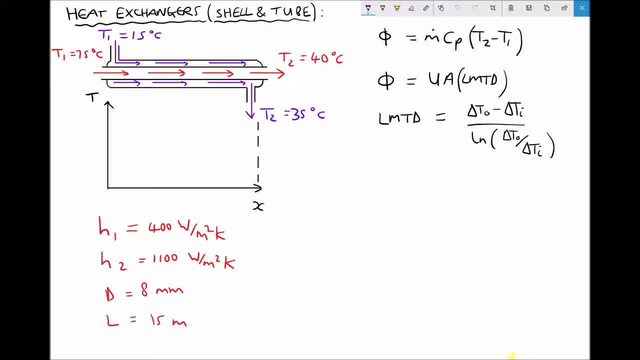 So underneath our diagram I've set up some axes, and on the y-axis is temperature and on the x-axis is distance along the heat exchanger, and we're going to use this in order to describe the two different classifications of heat exchanger: parallel and counter flow. Now the particular. 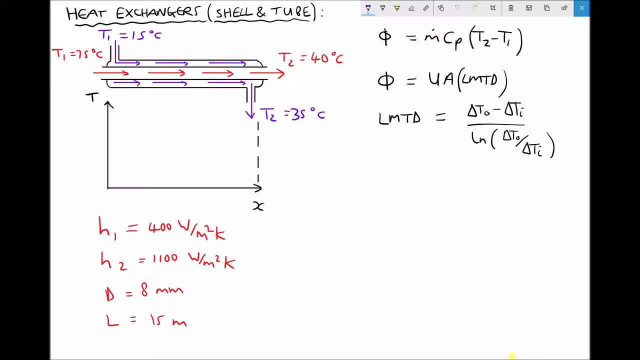 example that we have drawn here is a parallel flow heat exchanger, and we know that because the two fluids are traveling in the same direction from left to right. So let's make a quick sketch of the temperature profile for each of those fluids. Over on the left hand side we have the 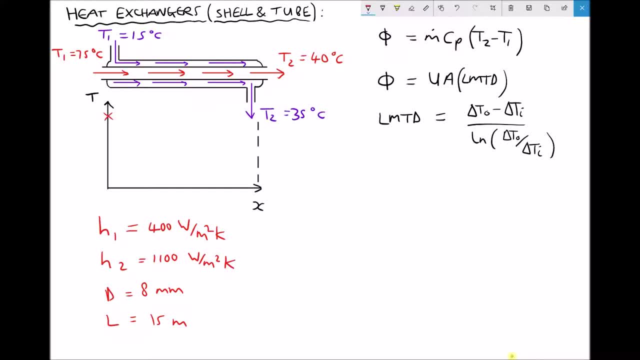 hot fluid starting at 75 degrees c and dropping to 40 degrees c, Like so. And our cold fluid starts at 15 degrees c and rises to 35 degrees c. So we end up with something like this Now: delta T O and delta T I for our log mean temperature. 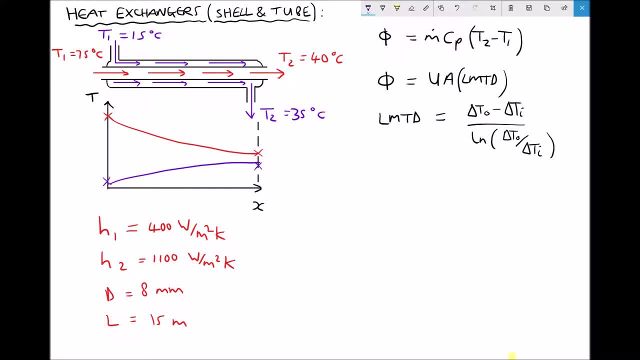 difference can be taken from this diagram, because delta T- I is the difference between our two inlet temperatures over here on the left hand side. So we can see that the temperature difference between our two heat exchangers will be about T- O. So first of all we've got to know what. 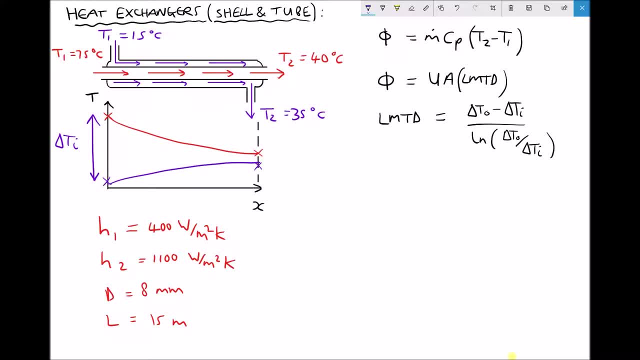 is the temperature difference between the two heat exchangers. Delta T O is the difference between the two outlet temperatures. So here we have delta T O. So first of all we are going to calculate delta T I and delta T O using the data given. Then we are going to 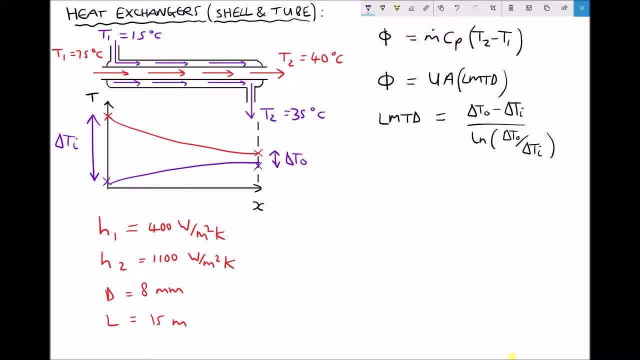 calculate U and A, and then we are going to calculate the rate of heat transfer through this heat exchanger. So, first of all, delta T I for our parallel flow heat exchanger is to be the difference between the inlet temperatures of our hot fluid and our cold fluid. Well, 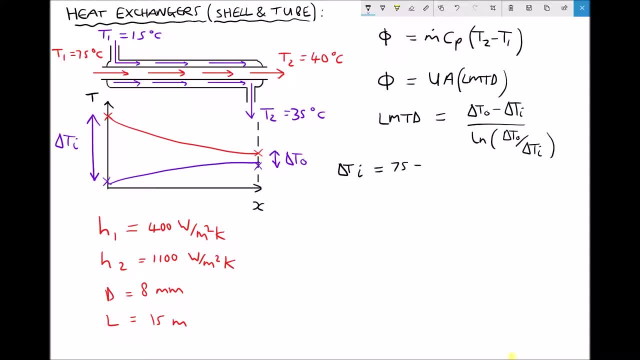 we can see the hot fluid at inlet is at 75 degrees C and the cold fluid at inlet is at 15 degrees C, giving us a delta T i value of 60 degrees C. We can repeat for delta T o and at the outlet we have the hot fluid at 40 degrees C and the cold fluid at 35 degrees. 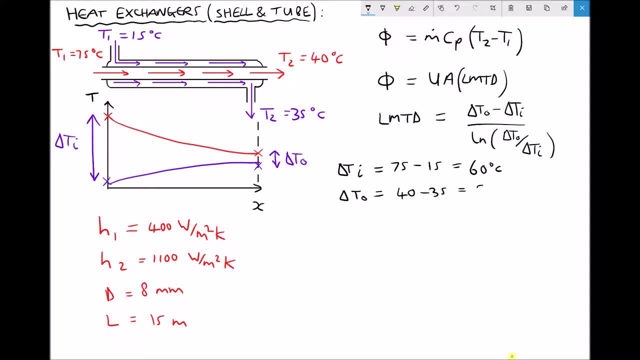 C. So 40 minus 35 equals 5 degrees C. Now, using that data we can calculate our log mean temperature difference. because our log mean temperature difference is delta T o 5, minus delta T i 60. Divided by the natural log of delta T o 5, over delta T i 60. Now, running that through, 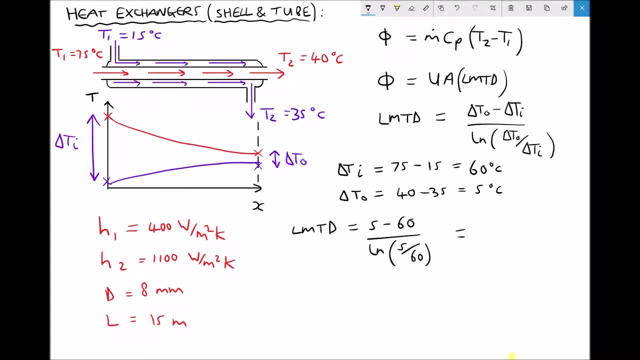 the calculator gives us a log mean temperature difference for the parallel flow heat exchanger equal to 22.134 degrees C, accurate to three decimal places. Next we can calculate our effective heat transfer coefficient, U, And the formula for this is relatively straightforward. We have 1 over U equals 1 over H1, plus 1 over. 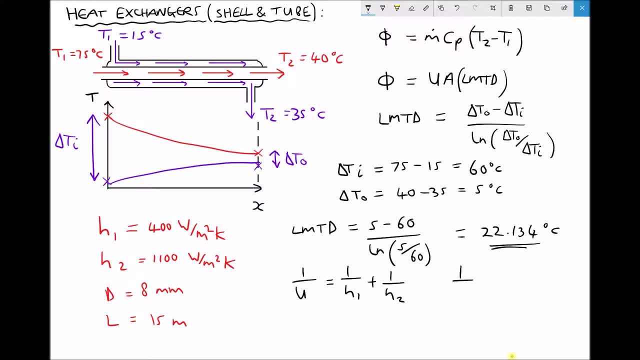 H2.. Therefore, 1 over U equals 1 over 400 plus 1 over 1100.. 1 over U equals 3.409 times 10 to the minus 3.. But note that it isn't 1 over U that we want, it's U. So if we do 1 over 3.409 times 10, 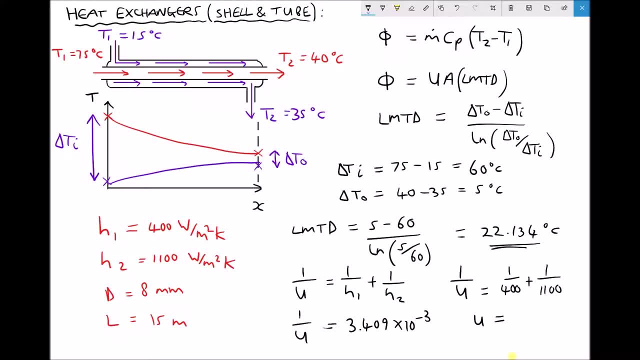 to the minus 3, we get a U value equal to 293.3 recurring, or 293.333 to three decimal places. That shares the same units as H Watts per meter squared Kelvin. Okay, let's transfer those values for log, mean temperature difference and U to the top. 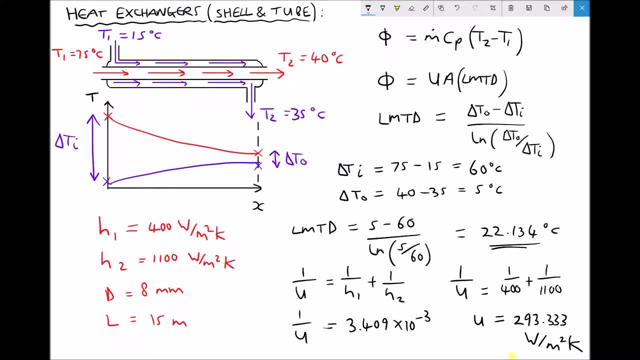 of the page and then we'll calculate the area and the rate of heat transfer. Okay, so, when it comes to calculating A, what we're actually calculating is the area that's in contact between the two fluids And, as we've already said, that's the outside surface. 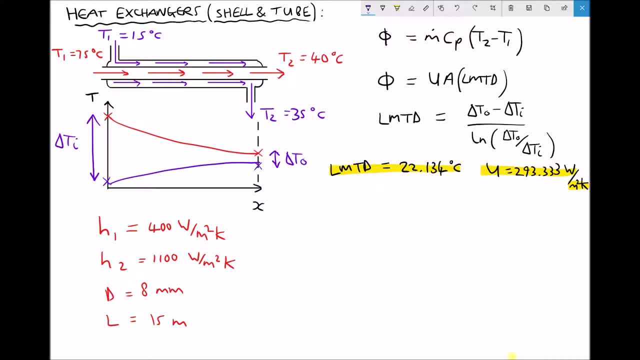 of the tube that runs through the center of the heat exchanger. So if we make a quick sketch, we can determine how we would calculate that area. So if this is the tube here, we need the surface area of the tube here. Now, as we've seen previously, the way that we would determine this is, we would imagine, 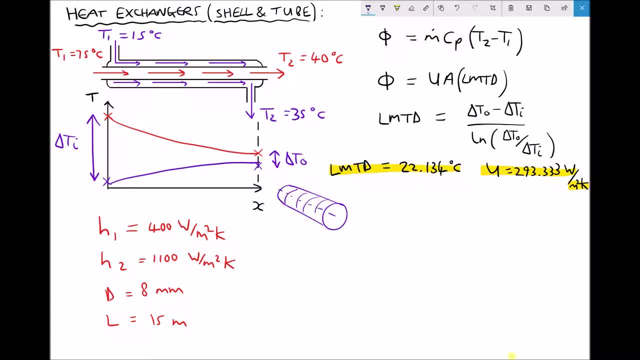 cutting down one side of the tube, like so, and then we're going to open it flat to form a rectangle. So, opening this flat, we have a rectangle and if we assume that this top edge here is the cut edge, Okay, So we're going to cut down one side of the tube, like so, and then we're going to open. 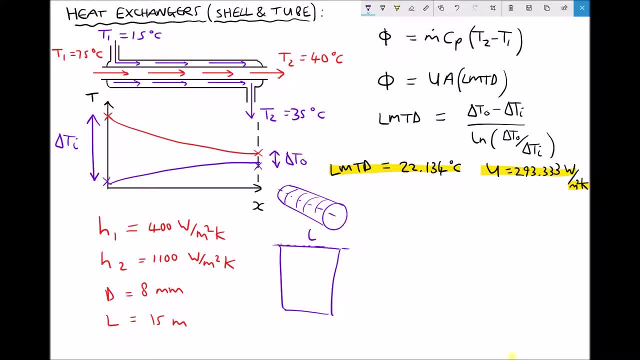 it flat to form a rectangle and if we assume that this top edge here is the cut edge, we're going to assume that that is going to be the same as the length of the tube. The other side of our rectangle represents the circumference of the circle and circumference. 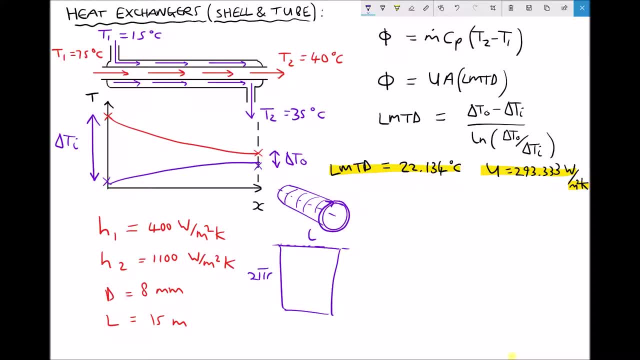 is calculated doing 2 pi r. Therefore the surface area in contact between the two fluids is 2 pi r times the length by multiplying the two sides of that rectangle together. So for the example we have given, the area is 2 pi r times the length. 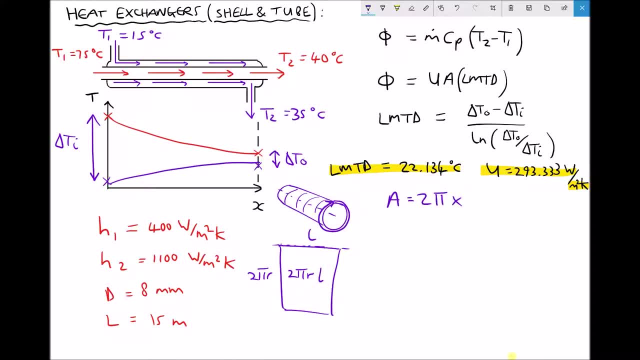 Well, the diameter is 8 millimeters, therefore the radius is 4 millimeters, but we need to express that in meters: 4 divided by 1,000 is 0.004, and the length of the tube is given as 15 meters. 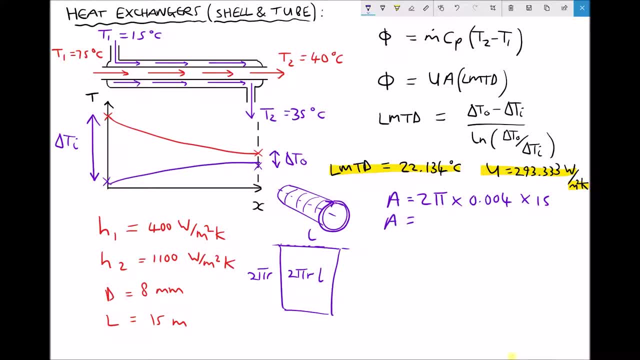 Therefore, the surface area in contact between the two fluids equals 0.3770 to 4 decimal places. Now, finally, we can calculate the rate of heat transfer, because the rate of heat transfer is the U value, 293.3 recurring times the area, 0.3770 times the log mean temperature. 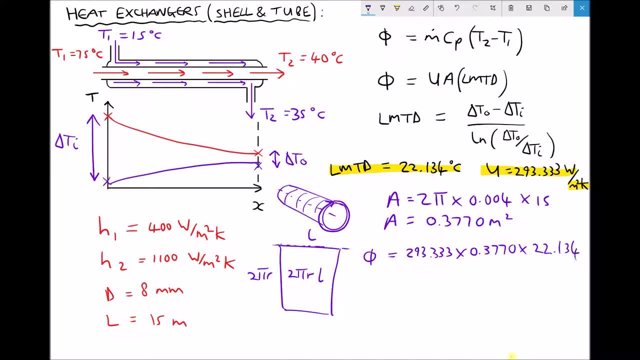 difference 22.134, giving us a rate of heat transfer through our heat exchange. So we're going to use that to calculate the heat transfer. So we're going to use that to calculate the heat transfer. So we're going to use that to calculate the heat transfer.